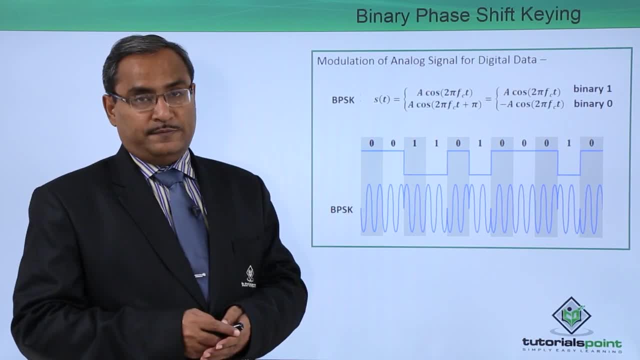 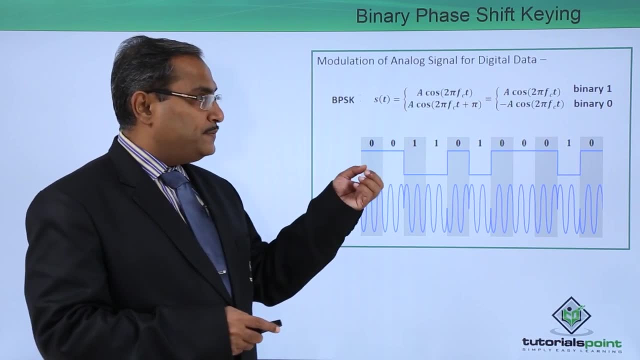 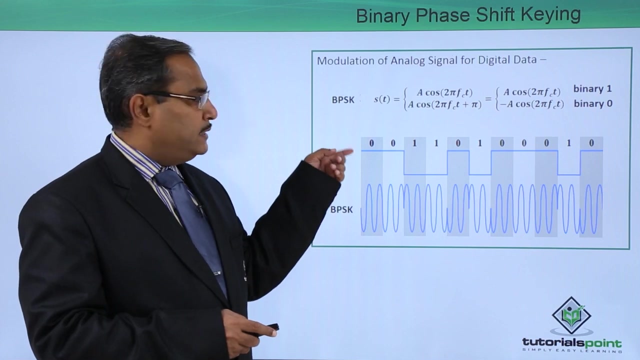 express it in the form that is: minus a cos 2 pi fct, So a cos 2 pi fct for the binary 1 and for the binary 0, it is a cos 2 pi fct plus pi. So here you can find that here we are having this respective binary inputs are there We? 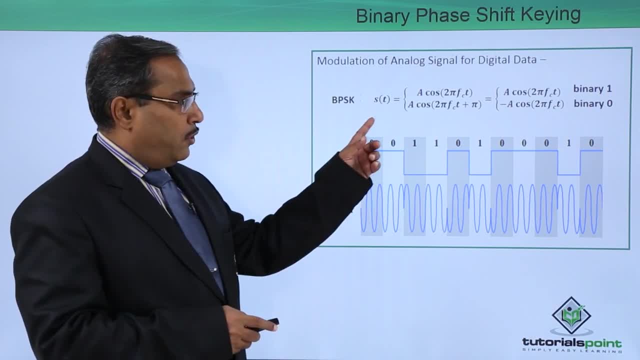 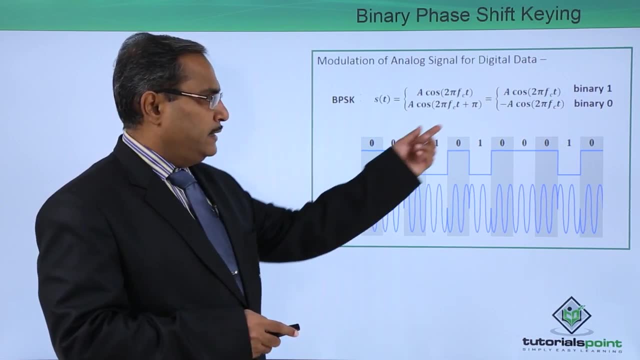 are converting it to the analog signal. So for binary 1, just, I am just for this- binary 0, we are having this respective waveform: are there? You can find that it is minus. So we have started this one from here and now we are getting this 0. So again it will. 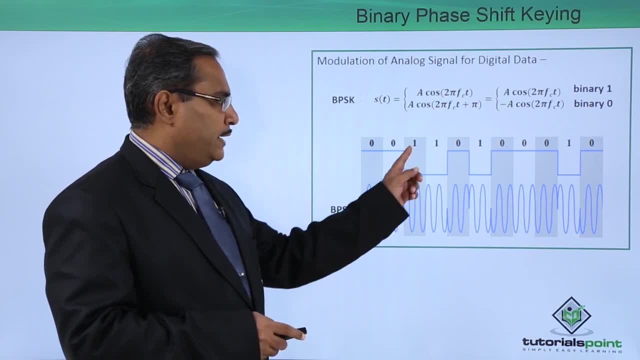 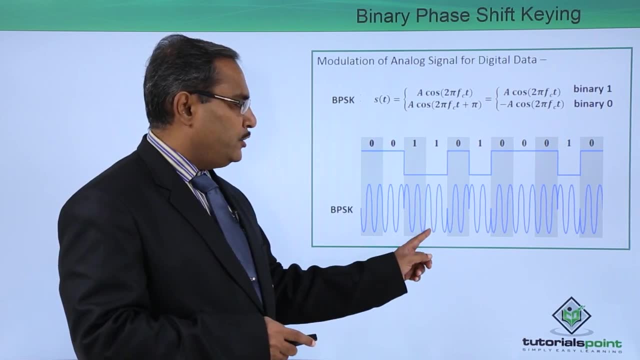 become negative, So it will be starting from here. So now, here it is 1.. So now it will be positive, So the phase shift will take place. Then it is 1. So the things will get continued, and as it is 0, so it will become minus a cos. 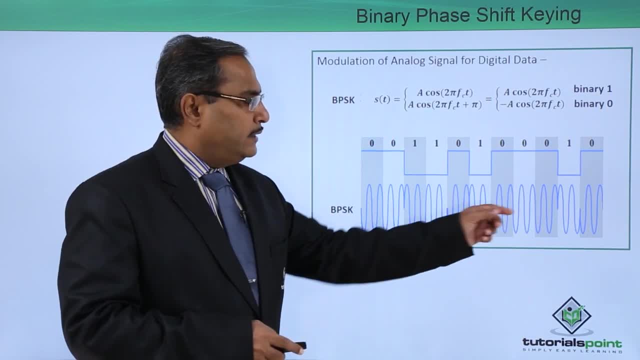 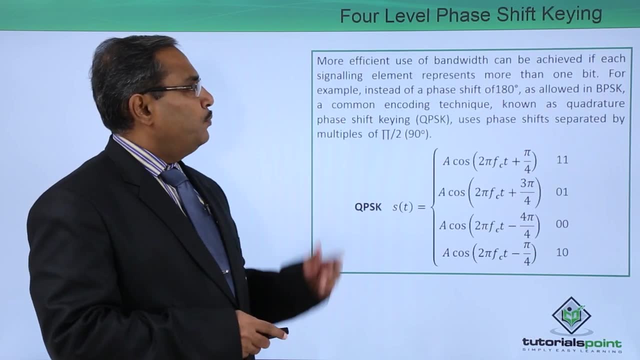 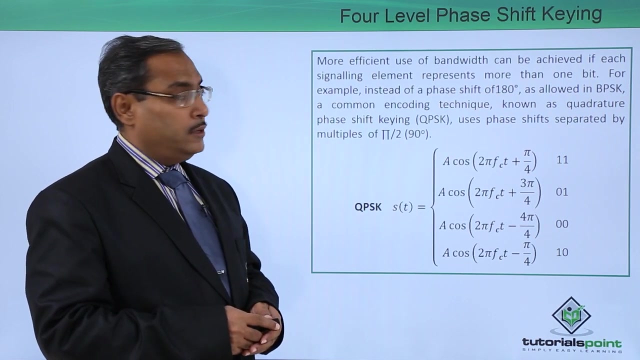 2 pi fct. So again it has become negative and the respective signal has got generated, and that is known as binary phase shifting. So more efficient use of bandwidth can be achieved if each signaling element represents more than 1 bit, But in the previous one we considered only the 1 bit. that is either 0 or 1, but that 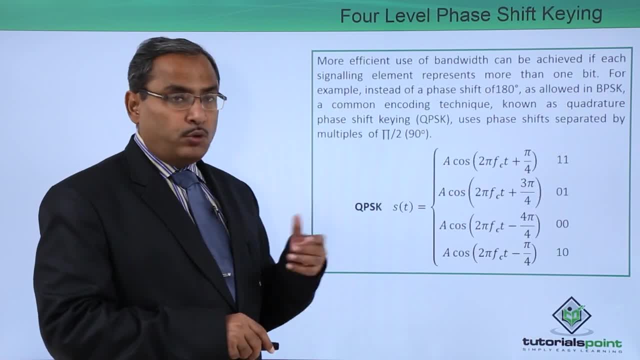 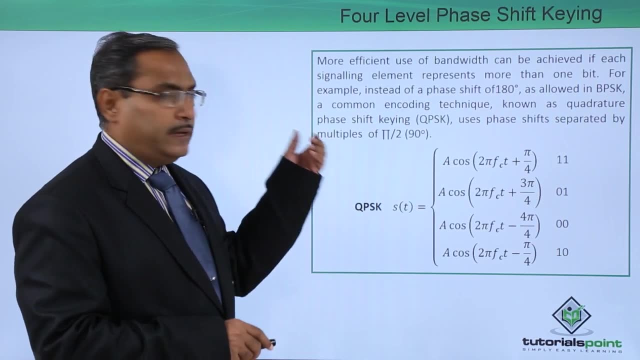 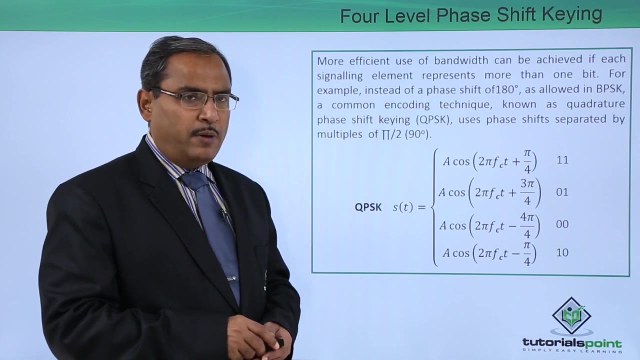 is a 0 or 1, we considered, but here, in this case, we will be considering more than 1 bits. For example, instead of a phase shift of 180 degree, as followed in case of BPSK, A common encoding technique known as quadrature phase shifting. in abbreviated form, it is: 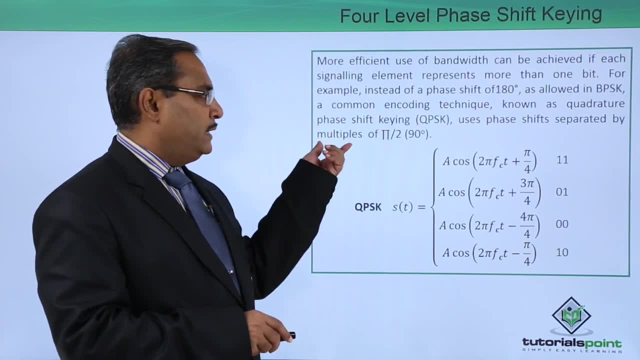 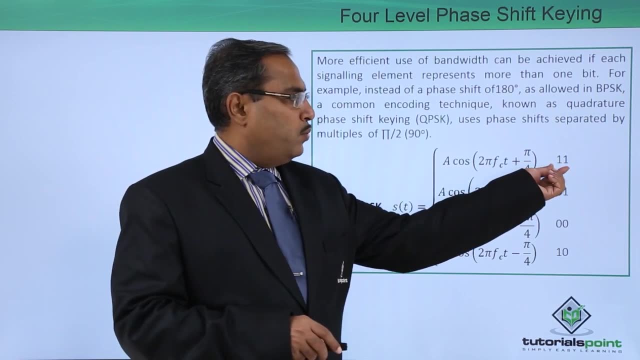 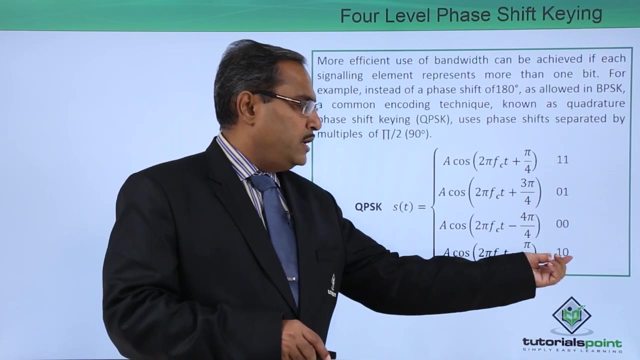 QPSK, which uses phase shifts separated by the multiples of pi by 2.. So the number of that is of 90 degree. So now for this particular bit pattern: 1, 1, this is the phase shift. for this 0, 1, the phase shift is given. for this 0, 0, this is the phase shift and for this 1. 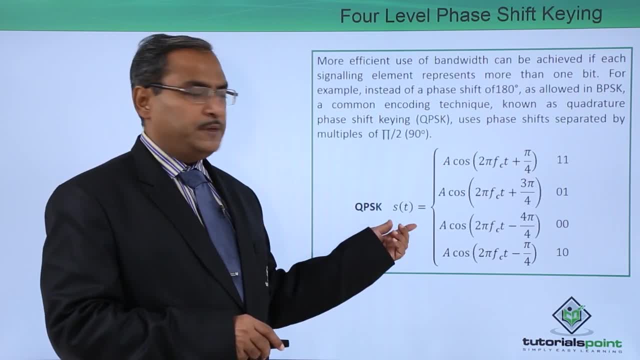 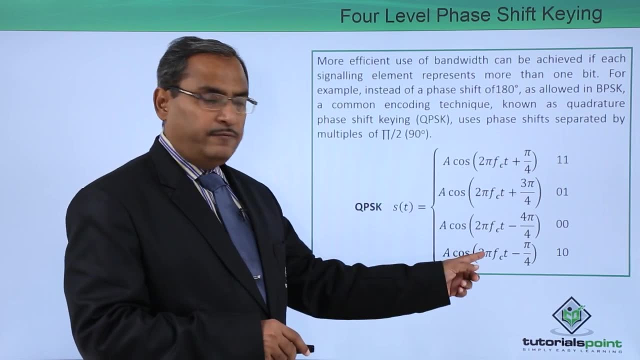 0. this is the phase shift and this is the modulating signals expression function. So here you can find that all of them are having the same amplitude, all of them are having the same carrier frequency. only the phases are getting shifted. So this is a good example. 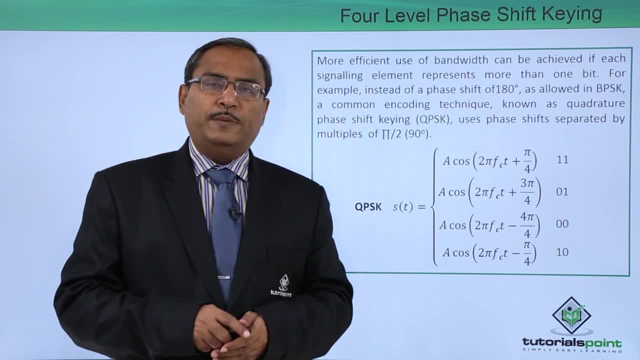 of 4 level phase shifting. So in this video we have discussed how this PSK is getting operated. Thanks for watching this video.